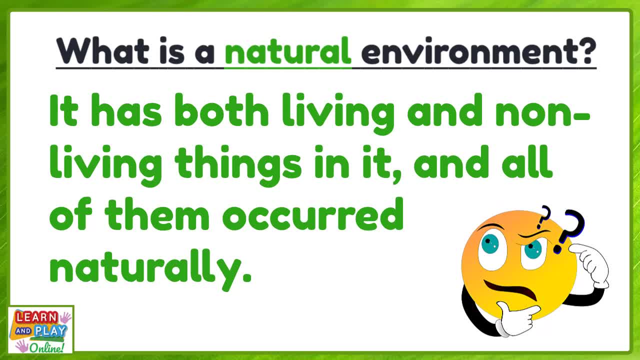 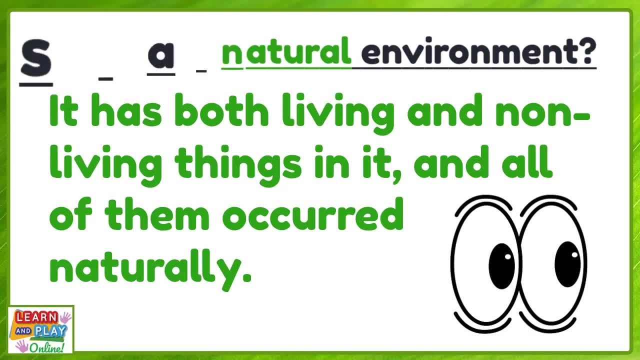 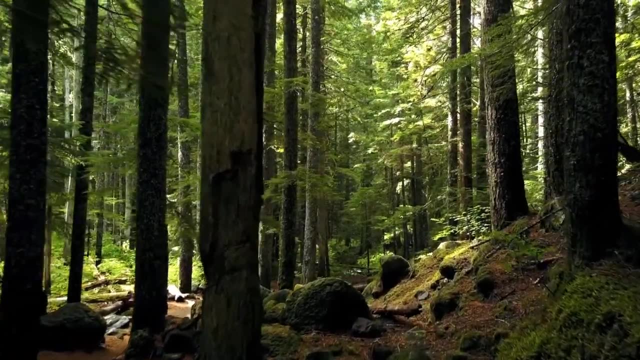 It has both living and non-living things in it, and all of them occurred naturally. Let's take a look at some natural environments so you have a better understanding. This forest is an example of a natural environment. All of the things that exist within this forest were created naturally, without the help of 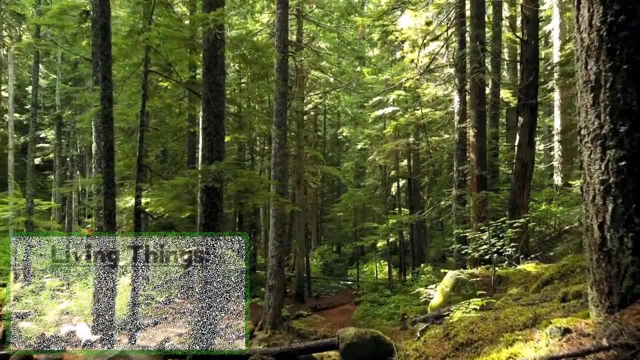 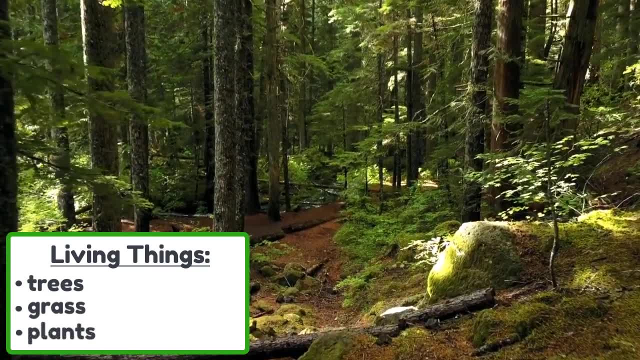 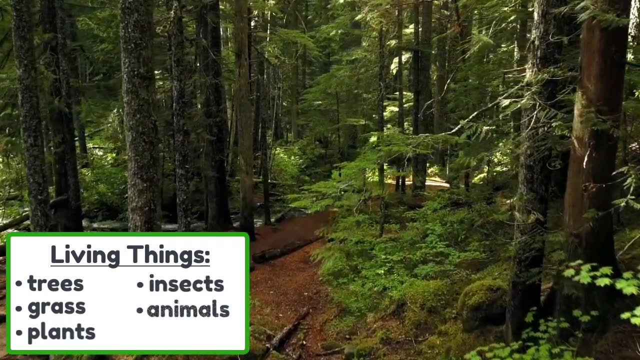 any human beings. You can see that there are living things in it, like different types of trees, grass and plants. There would also be other living things in this forest that we cannot see in the picture, including a range of insects and perhaps even some land and sea animals. 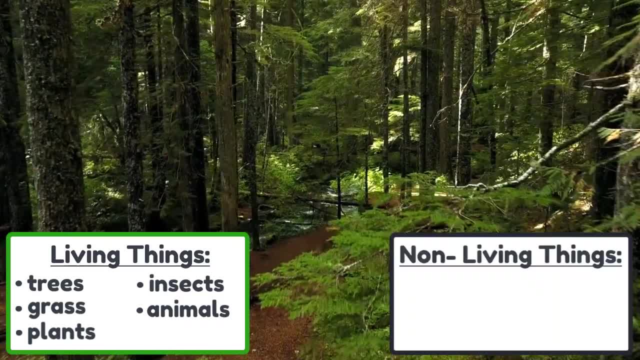 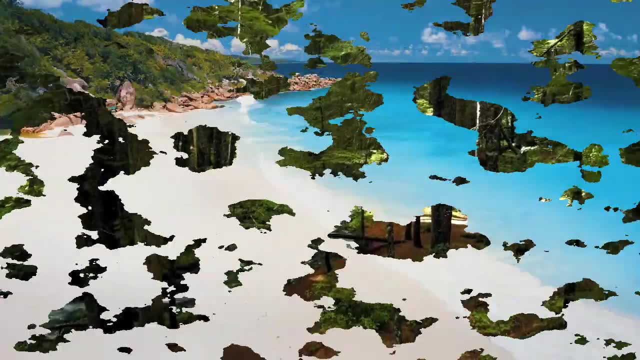 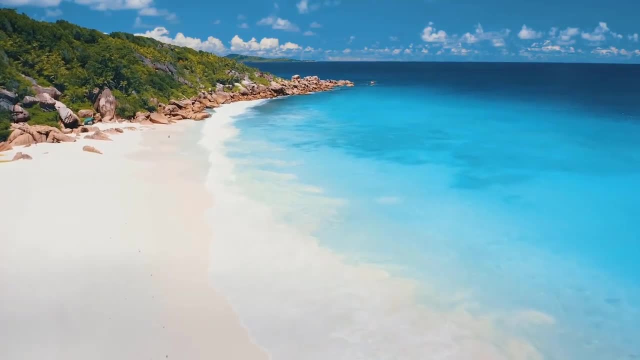 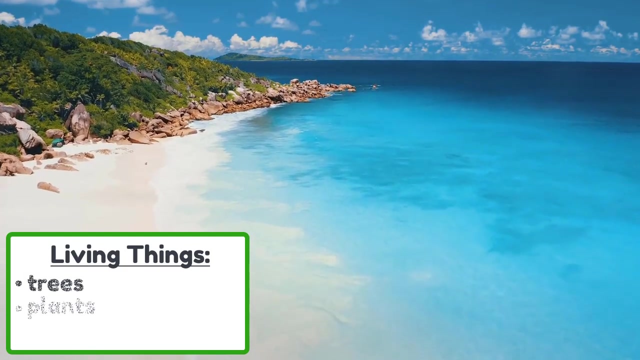 There are also non-living things in this forest too. These include the water, rocks and soil on the ground. The beach is another example of a natural environment. Beaches were formed naturally, as human beings did not build them. The living things that exist in this natural environment include the trees and plants. 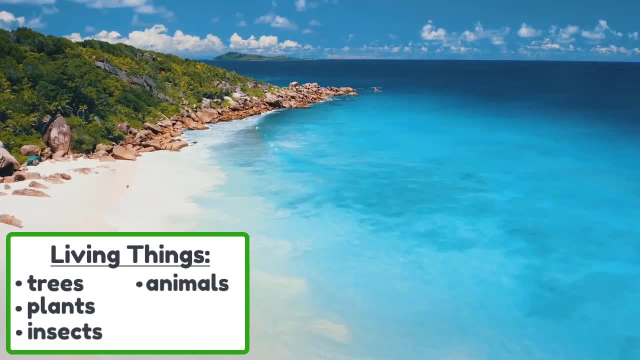 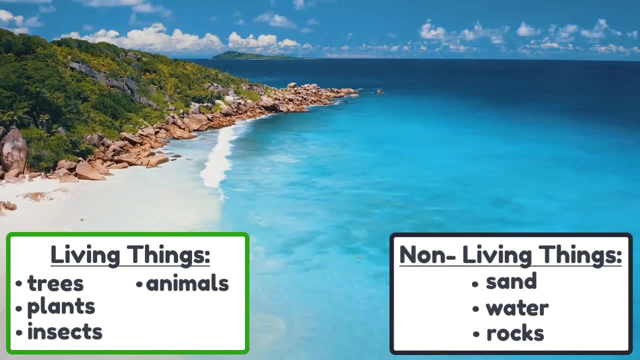 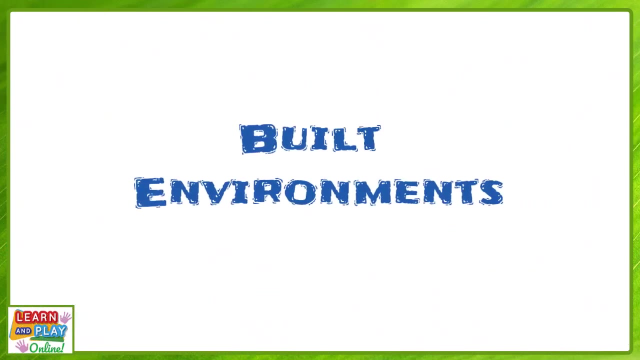 insects, and let's not forget the land and sea animals which we cannot see in the picture as well. Some non-living things include the sand, the water and rocks. Now that you have learned about natural environments, Let's move on to built environments. 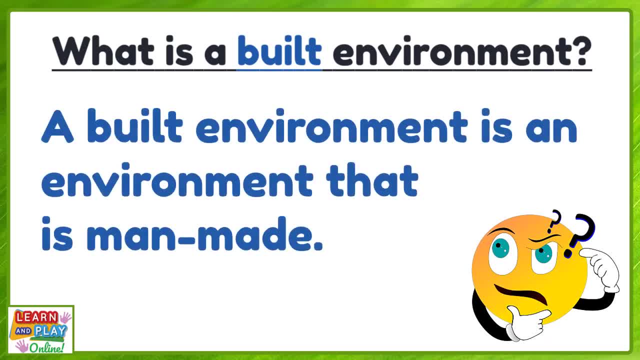 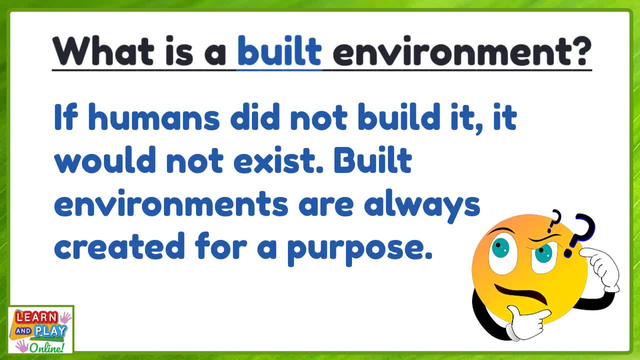 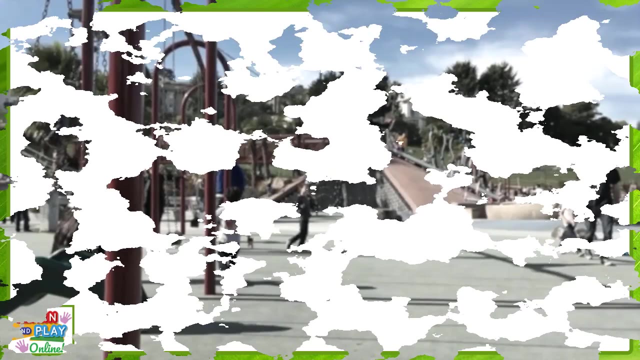 What is a built environment? A built environment is an environment that is man-made. If humans did not build it, it would not exist. Built environments are always created for a purpose. Let's have a look at some examples of built environments so you have a better understanding. 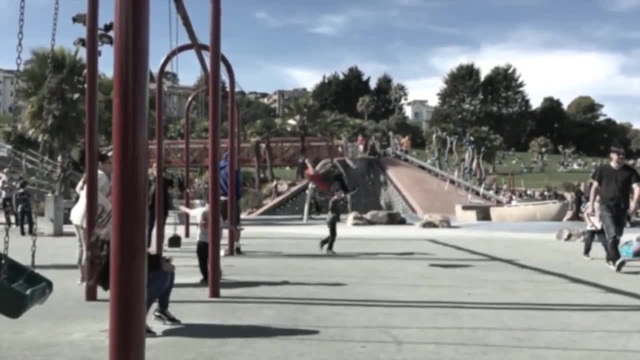 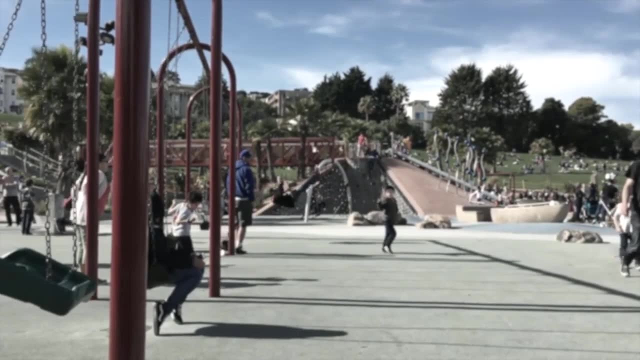 A built environment that you may often visit is a playground. Playgrounds are built to provide a space for children to play. Everything about a playground is man-made, including the design and equipment. There are also living and non-living things in built environments also. 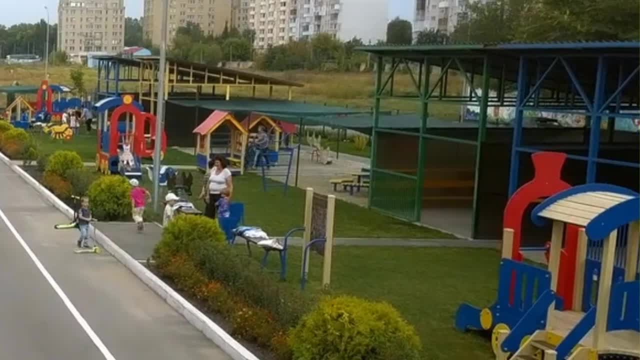 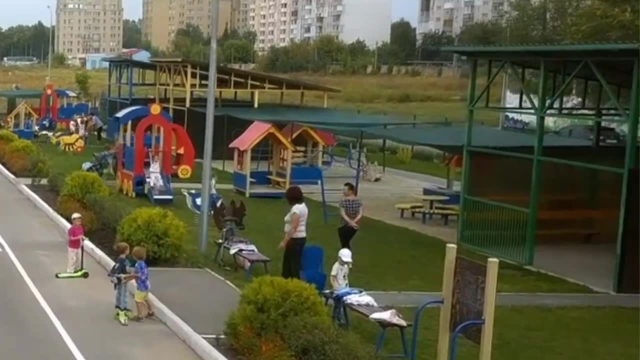 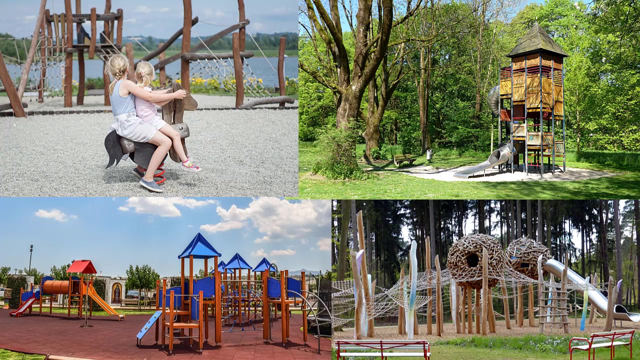 However, some living things, such as trees and plants, only exist in built environments, such as playgrounds, because they have been purposely put there as part of the design. Pause the video now to think about or discuss with someone about what a built environment is. Let's discuss about the living and non-living things that exist in a built environment, such 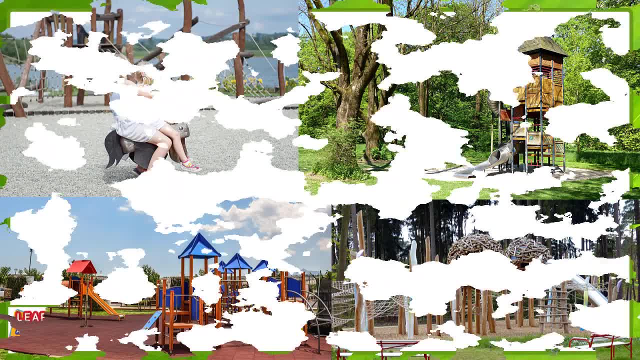 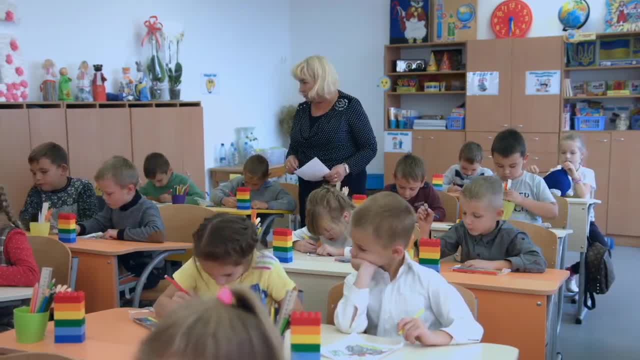 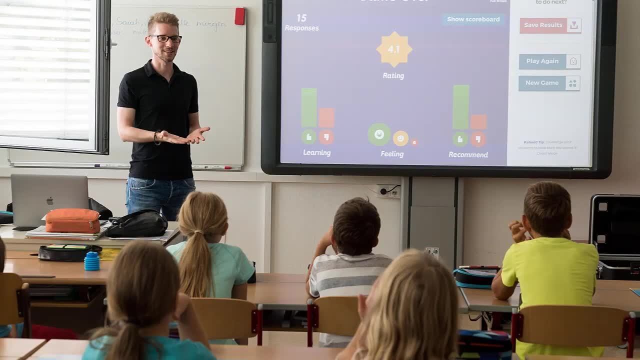 as a playground. Let's discuss a different built environment, one that many of you would know a lot about: A classroom. Classrooms may look different all around the world, but they have all been purposely built for a sole reason, and that is to provide a space for students to learn. 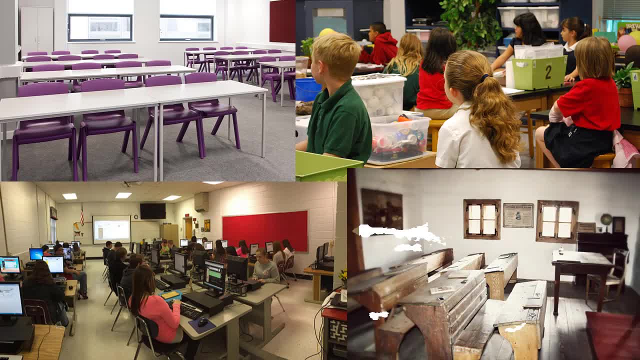 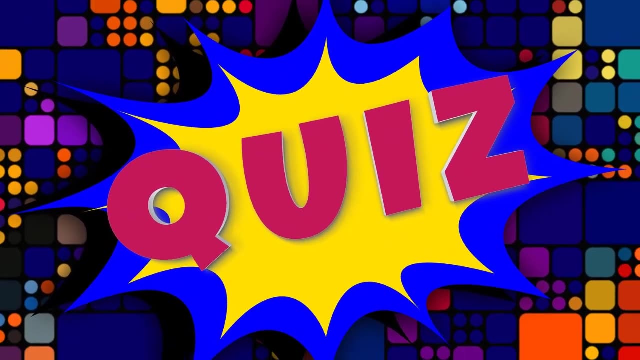 Classrooms are built environments because without human intervention they would not exist. That's why we call them built environments. Have a close look at the pictures of the classrooms. What living and non-living things can you see in the pictures? It's quiz time. 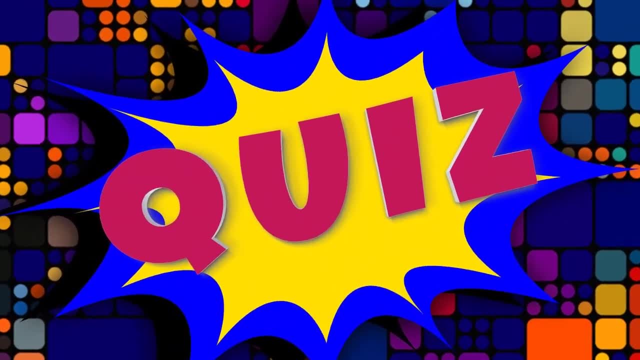 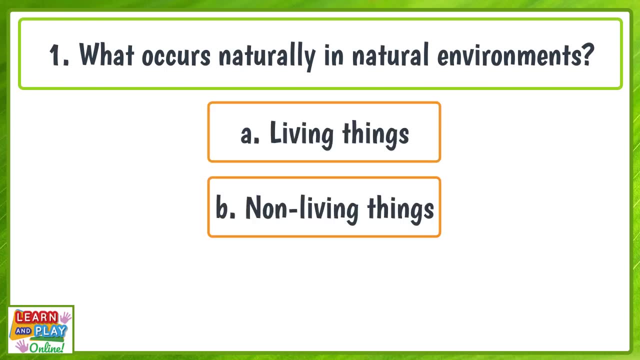 Let's see how well you've been listening. Question 1. What occurs naturally in natural environments? Living things, Non-living things, Both living and non-living things. It's quiz time. Let's see how well you've been listening. 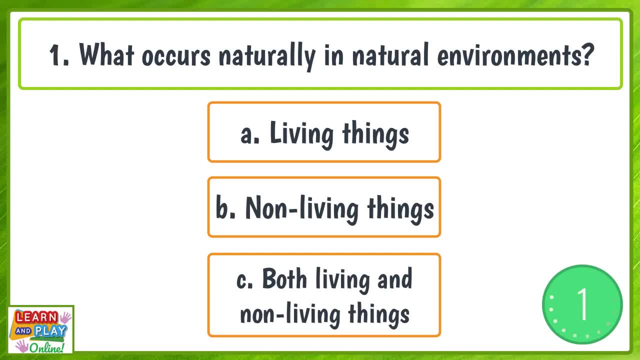 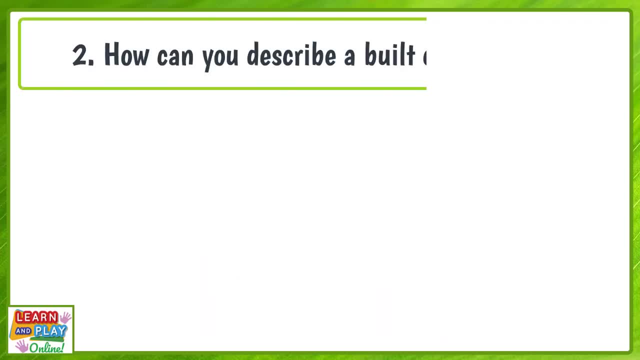 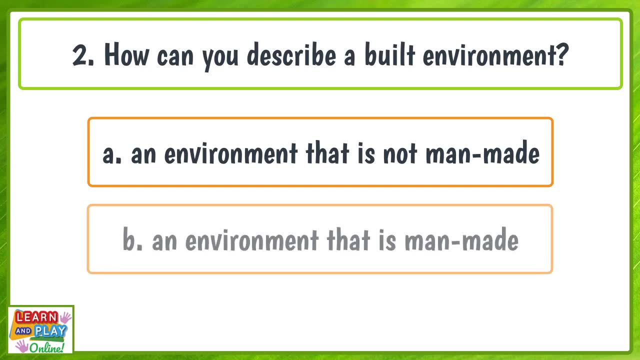 Question 1. What occur naturally in natural environments, Both living and non-living things? Question 2. How can you describe a built environment, An environment that is not man-made, Or an environment that is man-made, An environment that is man-made? 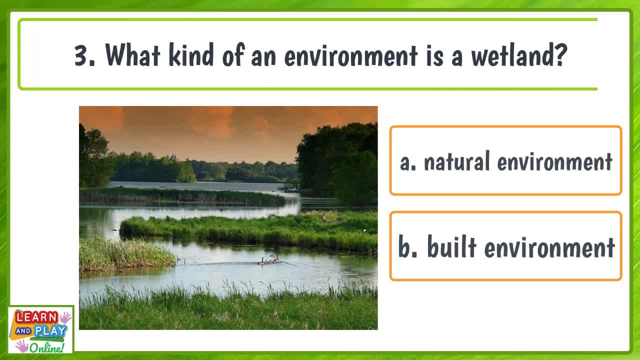 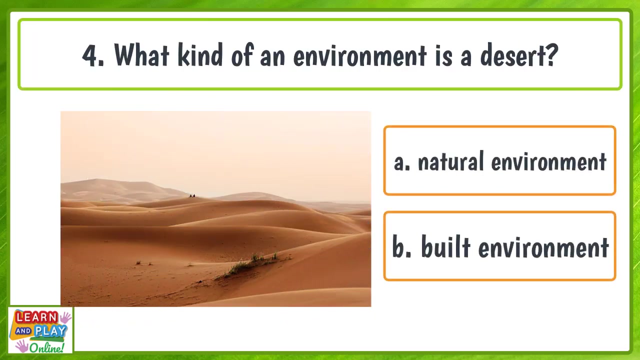 What is a built environment? A non-living thing. Question 3.. What kind of an environment is a wetland, A natural environment or a built environment? It's a natural environment, Question 4.. What kind of an environment is a desert? A natural environment or a built environment? 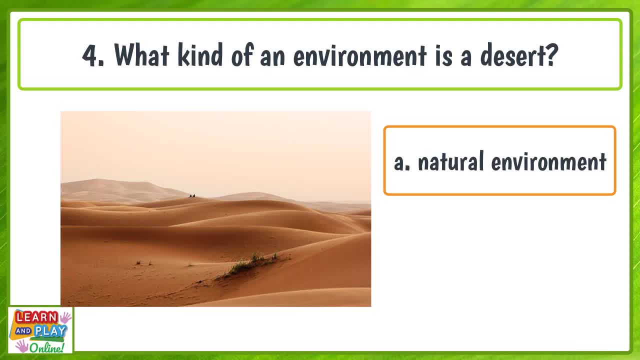 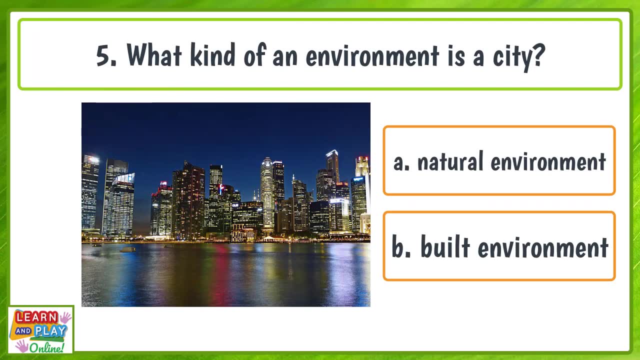 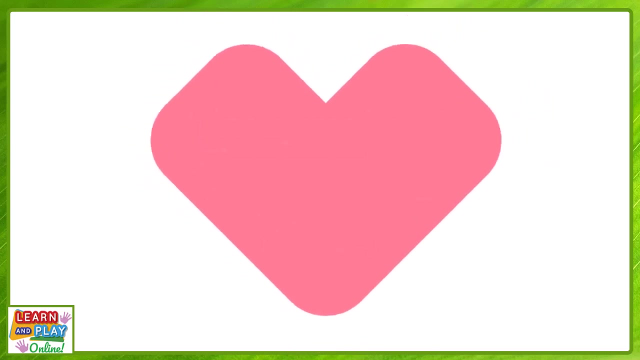 It's a natural environment. Question 5. What kind of an environment is a city? A natural environment or a built environment? It's a built environment, And that's the end of our quiz. How many did you get right? Question 6. What kind of an environment is a desert? A natural environment or a built environment? 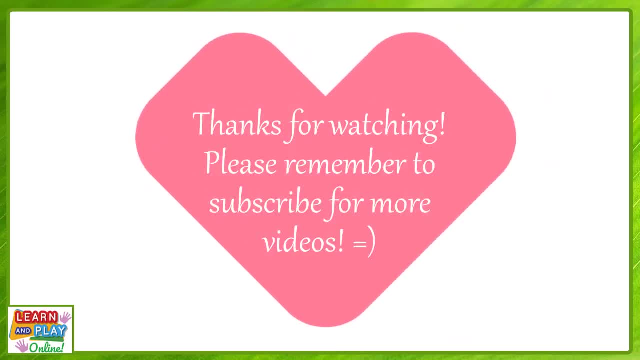 Thanks for watching. Please remember to subscribe for more videos.